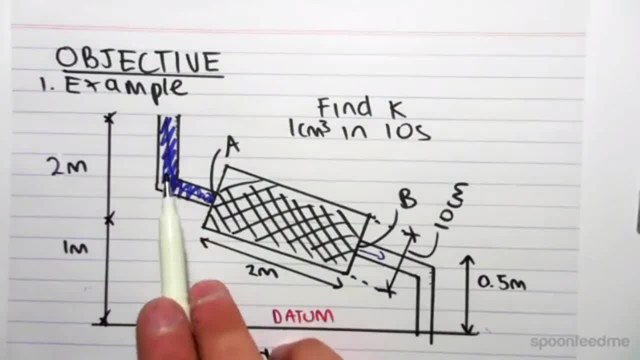 develop a pressure of water at a due to the height of the head. So we're going to have to divide that into the hydrostatic pressure. So because we're two metres below the surface at a this pressure, there's a pressure buildup of water. Now we know that pressure equals. 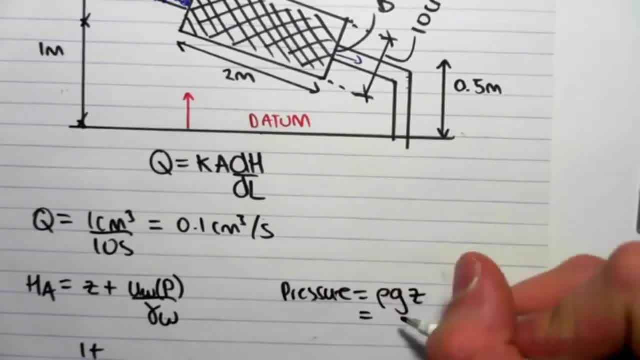 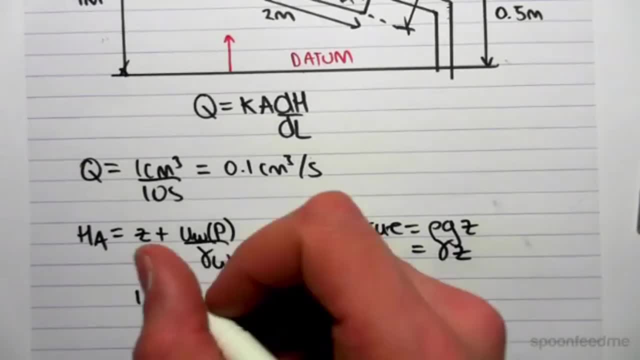 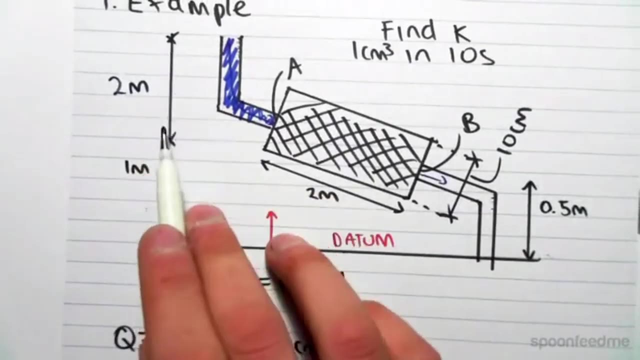 rho g, z, so that's hydrostatic pressure, which is the same as gamma z. Okay, So in our case the pore water pressure will be gamma z, which is nine point eight, one times by the depth depth. so we're 2 metres down from the top right, so it's times 2. on the gamma of water, 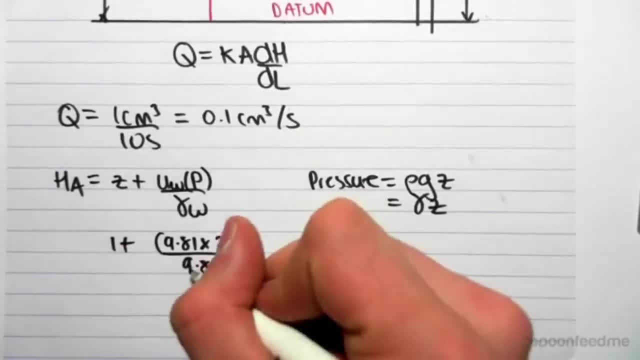 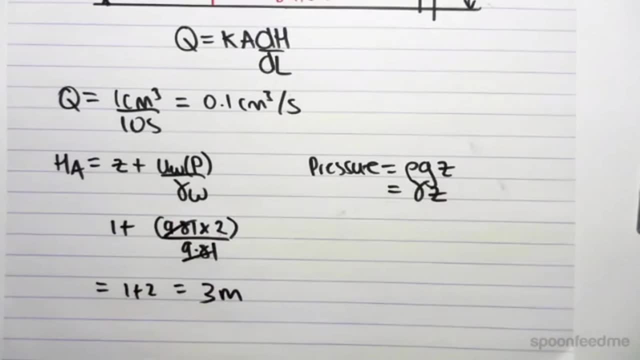 and the gamma of water is 9.81,. okay, so they're just going to cancel, which means we're going to be left with 1 plus 2, which is 3 metres. okay, so that's the head at A, the head at. 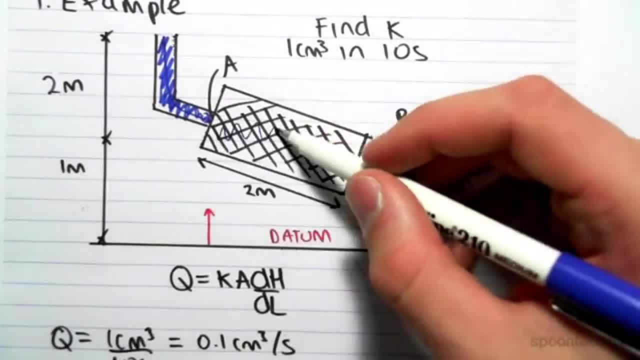 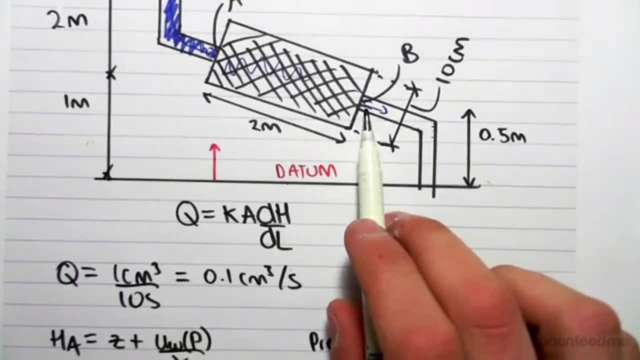 B now, because this water is taking its time to flow through. it's going to be like just dribbling out this end. okay, so there's actually going to be no build-up of pressure due to the water. the only thing that's going to cause flow is the elevation, so the head. 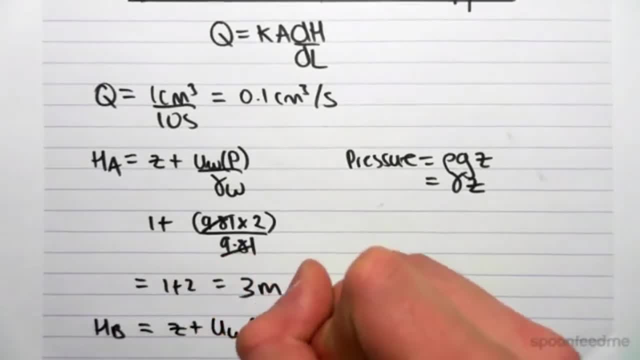 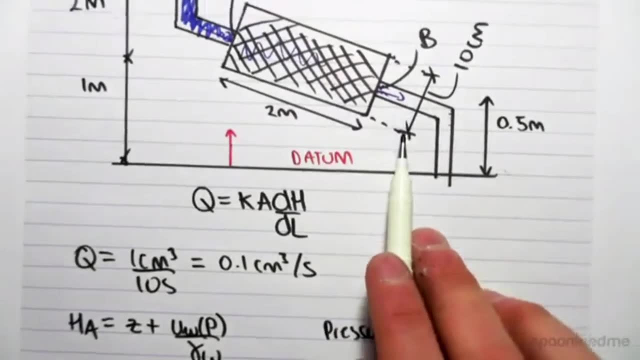 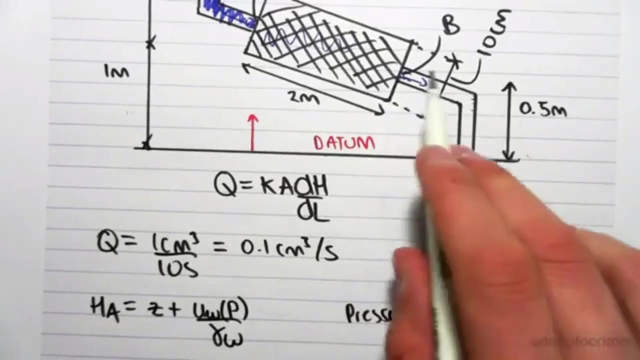 at B is Z plus the pore water pressure on gamma W. as we just concluded, there's no pore water pressure because it's just dribbling out, so there's no build-up of pressure due to water. there's just an elevation of 0.5 metres above our datum. 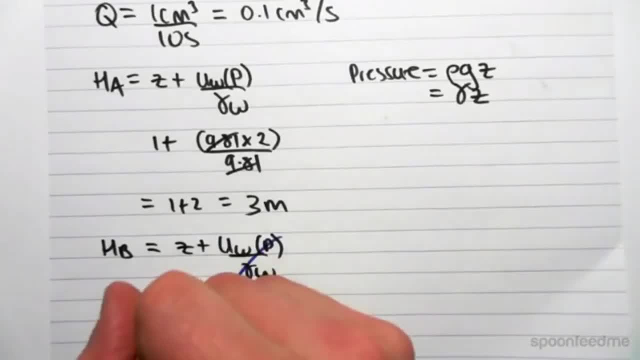 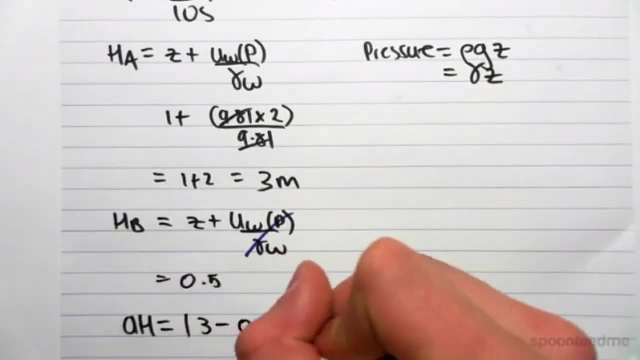 Okay, which means we can find DH, the change in head. we just use absolute values. you just want to know the absolute value. so it's 3 minus 0.5, which is 2.5 metres. okay now. 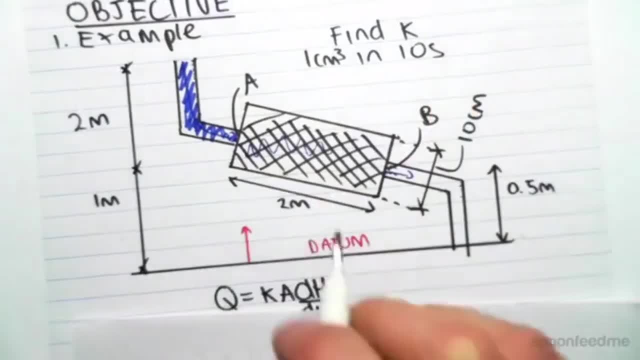 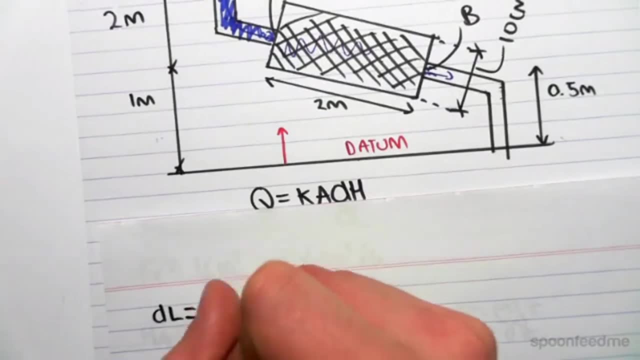 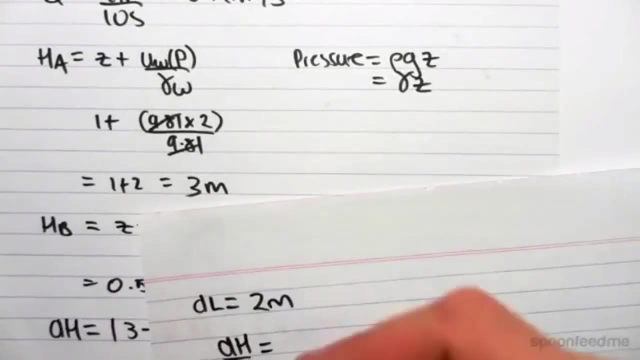 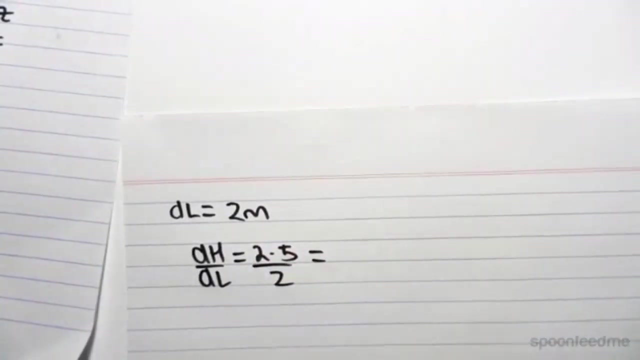 we can find DL, which is the change in length from A to B, which is simply 2 metres. so DL equals 2 metres, which means we can find DH of DL, the hydraulic pressure, which is the hydraulic gradient. so DH is 2.5 on DL, which was 2, and if we work this out, 2.5. 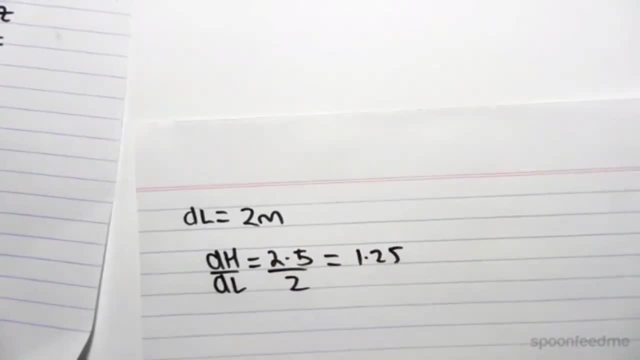 divided by 2, we get 1.25,. just also keep in mind that the units have to be consistent. 2.5 metres on 2 metres will cancel out, just to give us a number of 1.25, so we have DH.